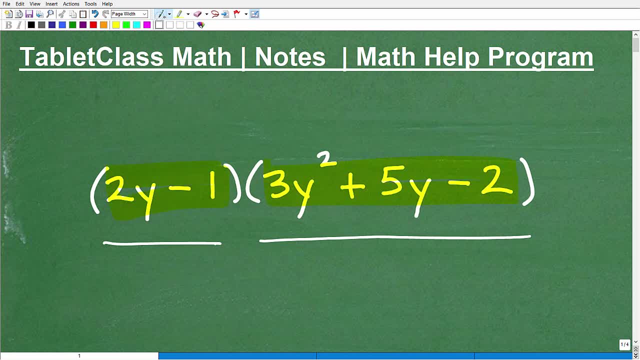 by a trinomial. So if you're studying algebra and you're, like, still not quite sure on how to multiply polynomials, well then this video is going to be very helpful to you And when you walk away from it, you're definitely going to have a happy face. You'll be like yep. 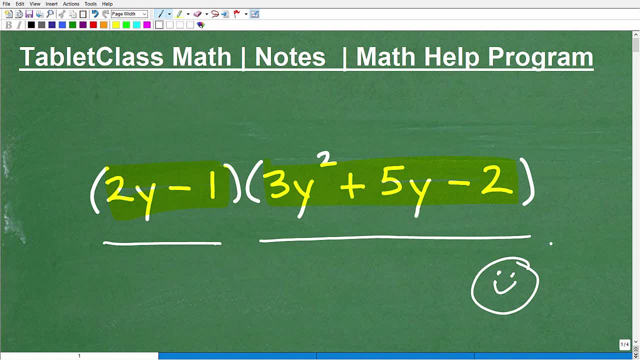 I'm ready for my quiz, I'm ready to impress my math teacher. Okay, so again a couple different approaches that you can take to multiplying polynomials. I'm going to teach you what I like to believe is, you know, kind of the easiest way to think about this. Okay, all right, so we're. 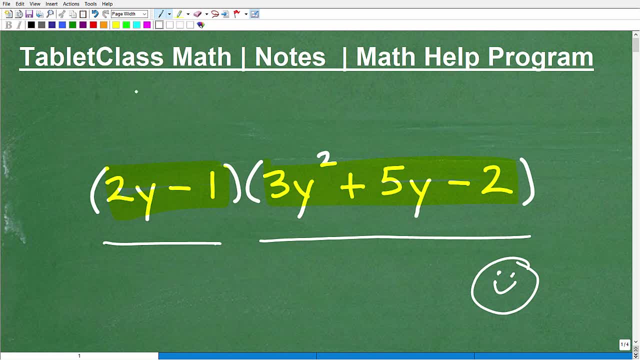 going to get to that in just one second, But first let me quickly introduce myself. My name is John. I'm the founder of Tablet Class Math. I'm also a middle and high school math teacher And over several years I've continued to teach math. And I've been teaching math for a long time And I've 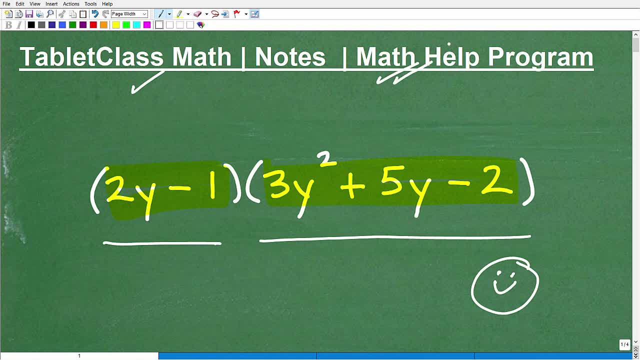 been instructing what I like to believe is one of the best online math help programs there is, But of course I'll let you be the judge of that. You'll find a link to my math help program in the description of this video, But basically I have 100 plus different math courses. I have all the 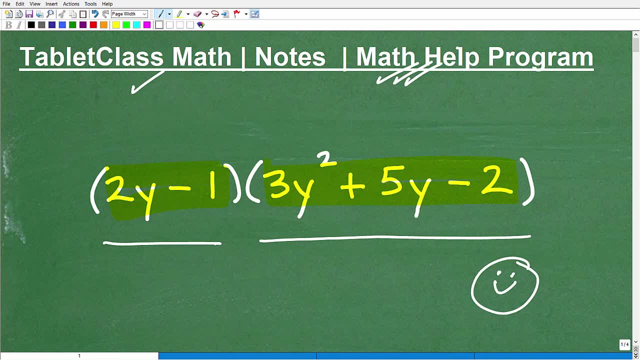 basic big courses like pre-algebra, algebra 1,, geometry, algebra 2.. I'm going to be launching pre-calculus here soon. I have college algebra, But I have many, many specialty courses, especially for test preparation. So those of you out there studying for, let's say, the GED, SAT ACT. 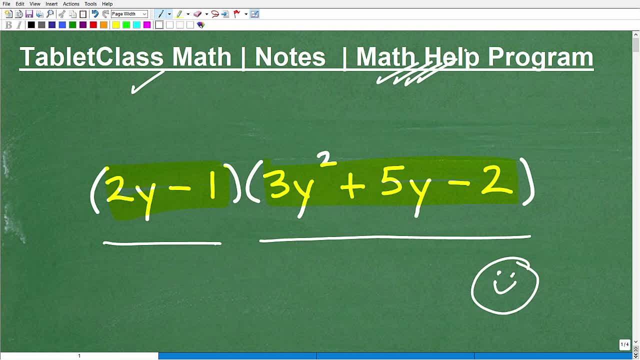 EASVAT you kind of get the picture: A teacher certification exam, nursing entrance, ACCUPLACER, ALEKS, CLEP exam. There's a lot of major exams that people have to take in life Very. 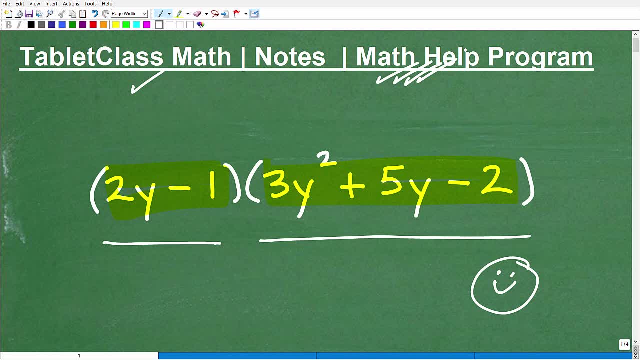 very important And these exams have quite a bit of math on it And again that could mean the difference between passing and failing. So I understand that there's a lot of people who need help in math to get ready for these critically important tests. So because of that I've developed 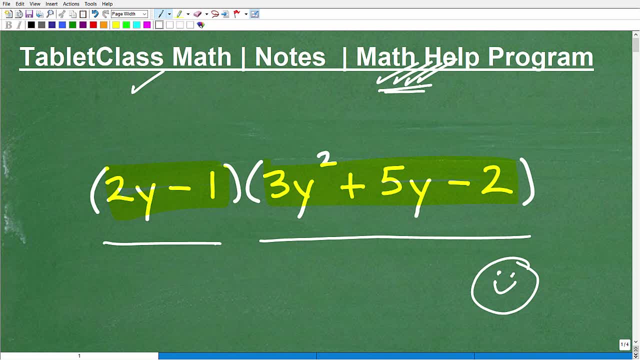 test prep courses. I've done a lot of work research on that. So, again, if you're you know, in that you know stage of your life where you're studying for one of these tests, go to my website and see if I have your exam. If I don't, drop me a line in our contact form and I'll see what I can. 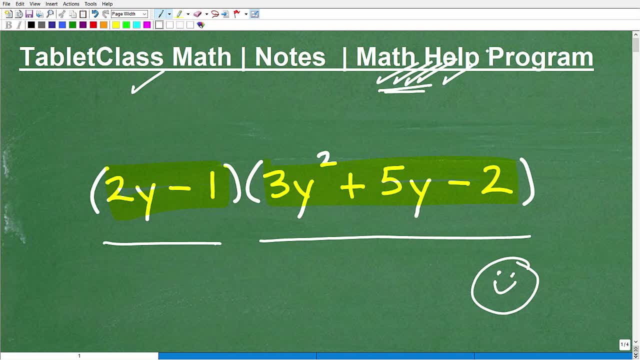 do? I also help those who do like independent study, like homeschoolers, have a complete, full curriculum and a nice homeschool program, And obviously I help those that are struggling, struggling in their current class. So if you're taking algebra, algebra two, whatever the case is, 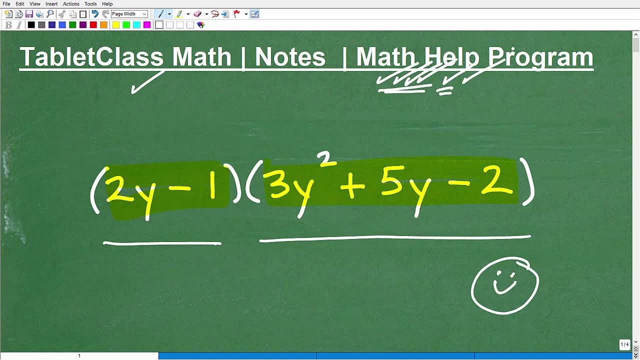 pre-algebra and you're- just you know- struggling and you need more instruction, more practice, more clarification on this. obviously, my program can help you out, But if you want to start helping yourself out immediately, you need to take a great math notes, Okay, And over decades of teaching. 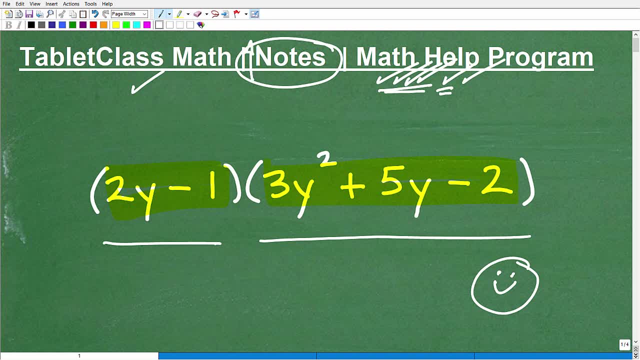 math. this is like my golden rule And I've seen it just time in and time out. Those students who take great math notes almost always like looks like this person. At the end of the year they have these awesome grades, A, plus, 100%. They're walking around, or. 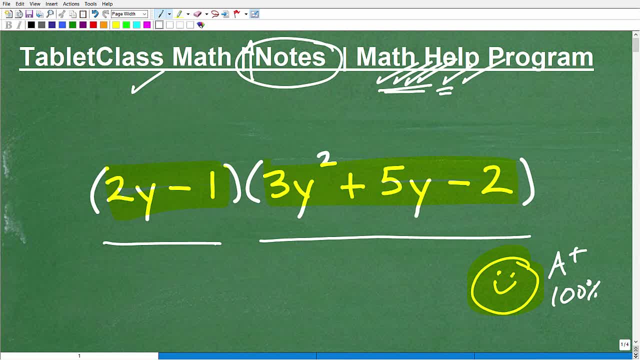 like: look at me. I you know I'm a superhero because I got this A in algebra. You know it's always nice to get a nice grade. but the reverse is true. Those students who just don't take notes in class- you know take sloppy notes- might occasionally take notes like to look at. 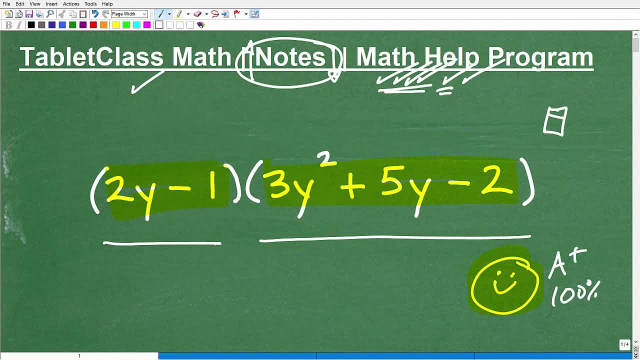 their cell phone, you know, maybe like to talk to the person next to them or rely on their best friend, who takes far better math notes than they do. Listen, I get it. I'm not a math nerd. I'm not a math nerd. I was a student once And, trust me, if there were cell phones back in my day, I don't. 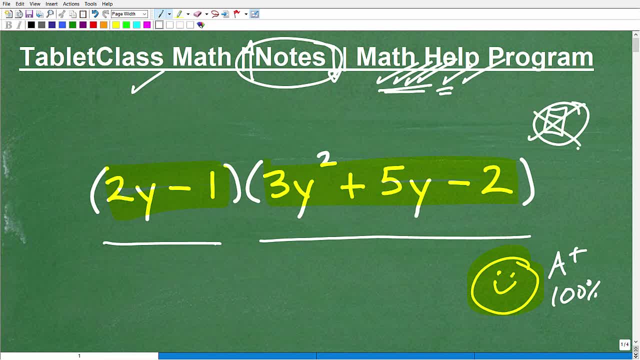 even think I would have maybe graduated right, Because cell phones are completely distracting. All right, This technology, listen, I know it's useful, but you have to be super focused if you're going to learn math. It's just too much information Okay, And note taking keeps you focused, Not only. 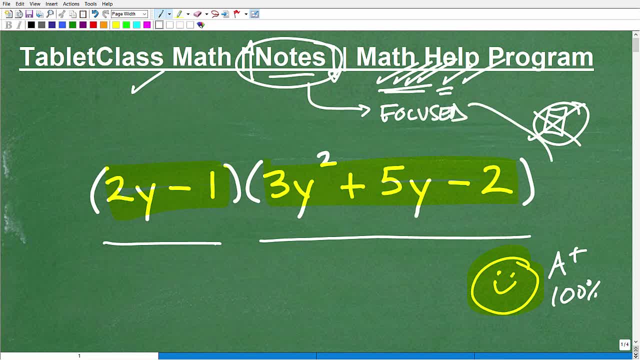 does it keep you focused? it is going to help put that information into your brain. Okay, Retention, comprehension, Okay, The mechanics and the process of you taking notes, great notes- is just going to help you. so just so much, All right, So please improve your note taking if this message applies. 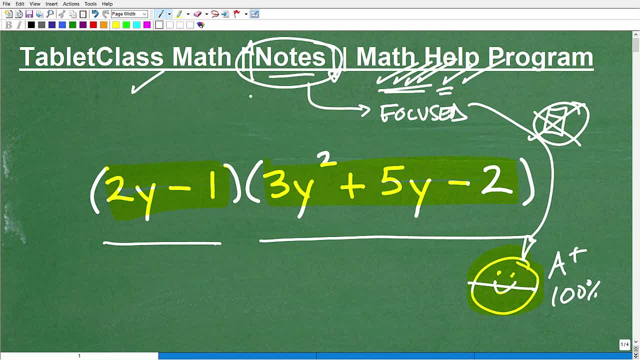 to you, But in the meantime you need something to study from. So I offer detailed, comprehensive math notes to include pre-algebra, algebra one, geometry, algebra two and trigonometry. You can find links to those notes in the description of this video. All right, Let's get into multiplication. 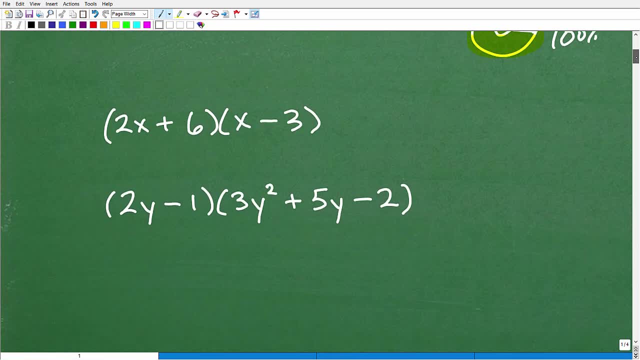 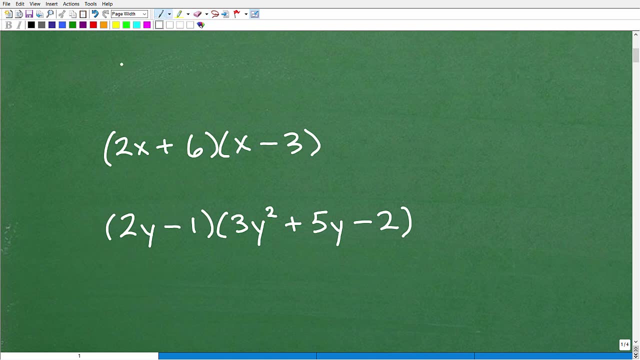 of polynomials and let's take a look at some basic. let me get rid of this little figure there, so we have some nice, clear way to think about things. Let's take a look at these problems. Actually, I'm going to add one. 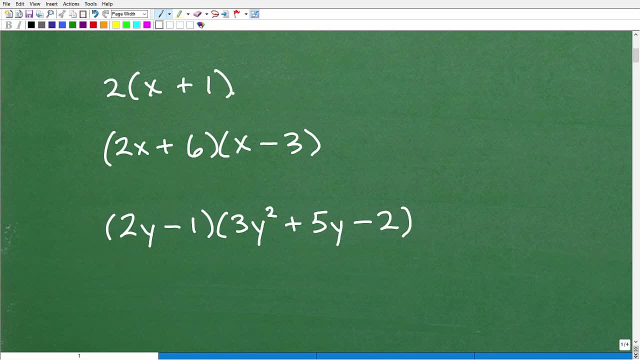 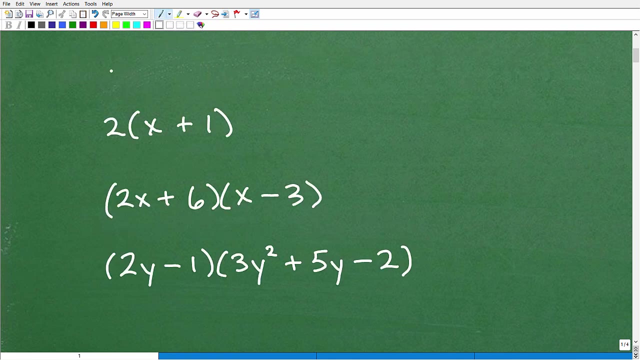 in here. Okay. So here, when you start learning how to multiply polynomials, okay, you're going to start off with a problem, something actually. let's even add another one in here. Okay, How about this x times 4x? Okay, So here we have three different, four different problems And obviously we're going. 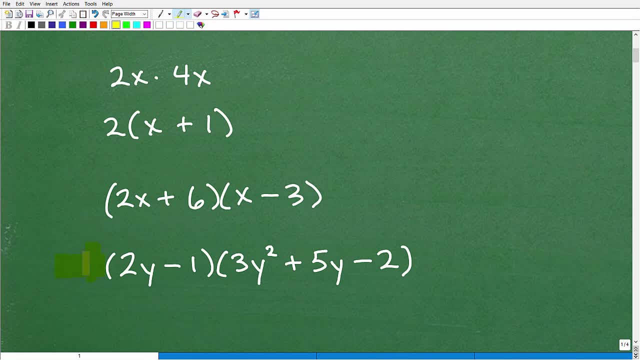 to do the problem right here that we're interested in. Okay, Now, if you want to kind of check for your understanding, to see if you know how to do these problems, you know go ahead and you know, pause the video and knock this out, maybe turn this into a little quiz, But these, all these here, 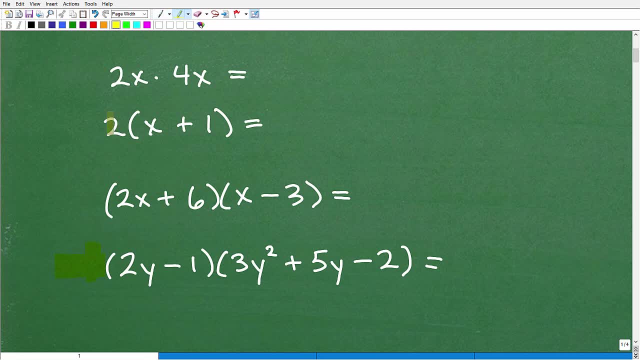 are polynomials. Now, this is a number, okay, but technically you can kind of consider it a polynomial, But let's start with a number. So let's start with a number. So let's start with a number. Let's just review. Okay, Let's make sure you can do these more basic problems before we do this. 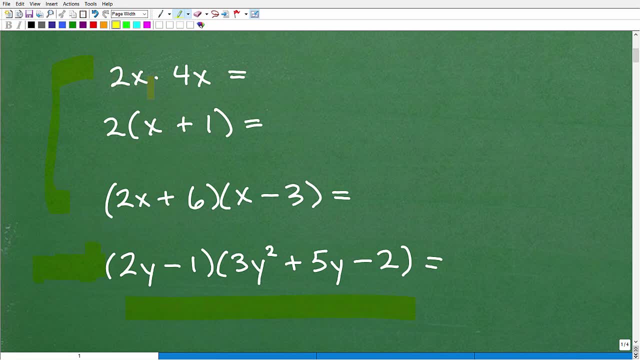 kind of more advanced problem. All right, So 2x times 4x- Okay, How do we do this? Well, we're going to multiply the coefficients together. So 2 times 4 is 8.. And then x times x, we're going to. 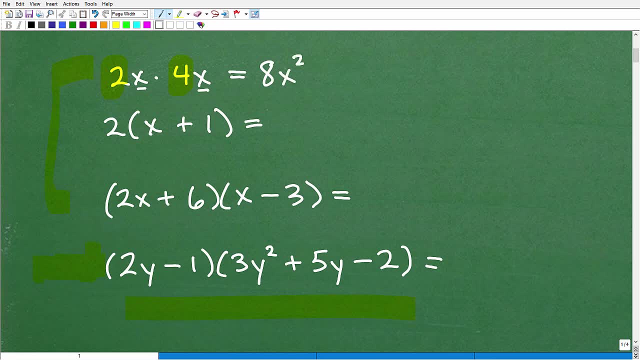 multiply the variables together, is x squared. Okay. So if you got that right, give yourself a check and give yourself a little smiley face. Okay, How about this next problem? All right, Let me scoot this down. Well, this problem is going to require you to understand the 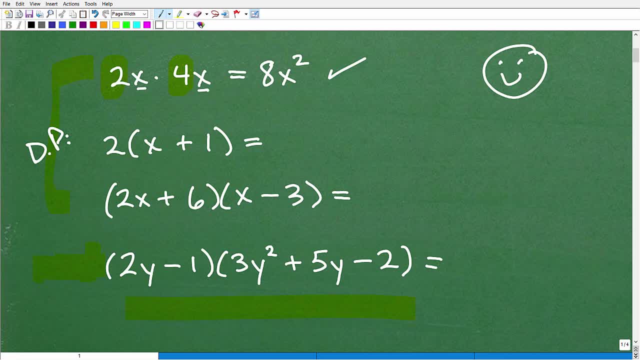 distributive property, And this is really, really a weak area for a lot of students. Okay, So what we're going to be doing is we're going to distribute: okay, this 2 to this x and this 1.. All right, We're going to multiply. Okay, This 2, let's actually run it out. That'll be 2 times x. 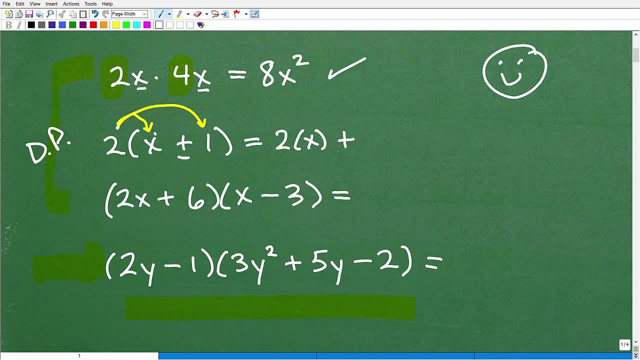 All right, 2 times x plus this is the plus 2 times 1.. Okay, So you got to know the distributive property. So 2 times x is of course 2x, And 2 times 1 is of course 2.. So this is 2x plus 2.. Okay, So if you got that right, give yourself a. 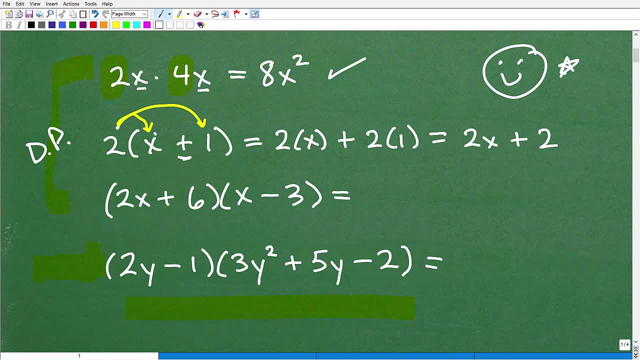 little star. Very, very good. All right, Now we're going to move on to this guy right here: 2x plus 6 and x minus 3.. Hmm, How do I do this? Well, actually I'm going to do this problem here. 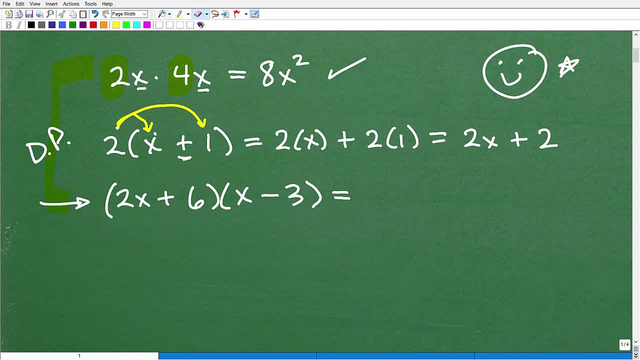 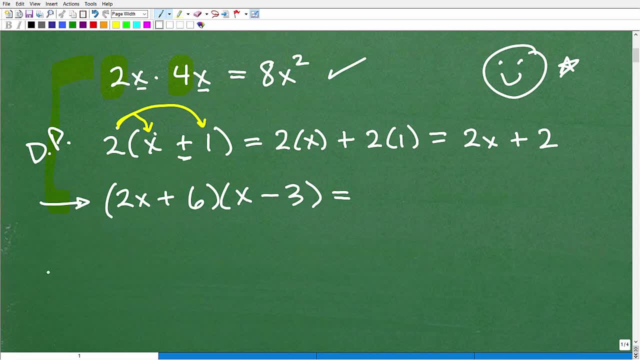 problem All right. So that's the question. Well, if you're thinking the FOIL method all right, then you're on the right track. This problem generally when you're introduced to how to multiply a binomial times another binomial. okay, here we had a number times a binomial And then 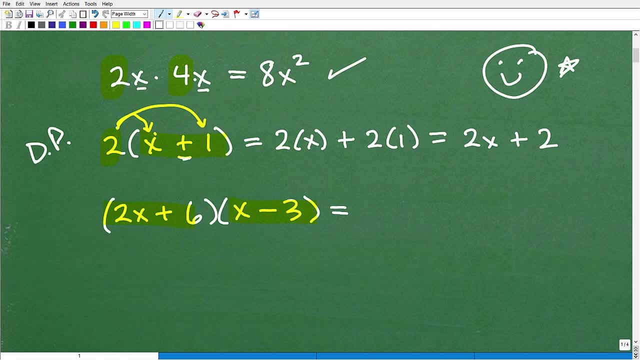 we had. these guys are called what Monomial, So monomial times a monomial, And then we have a binomial. But now we got a binomial times a binomial. So how do we do that? Well, typically most students are taught the FOIL method And the FOIL stands for first, outer, inner, last. So how? 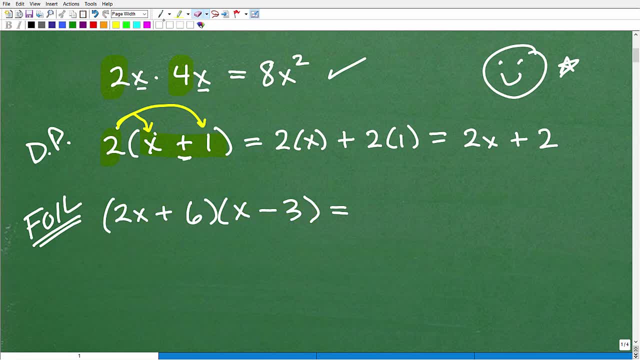 does that work? Well, let's go ahead and do this now. So here these guys, right here are the first terms of these binomials. Okay, So that's the first part. Okay, In fact, let me just erase all. 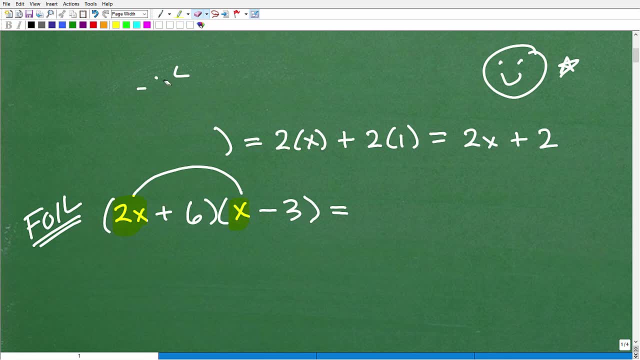 this stuff here so we can Really concentrate on the FOIL method, And this is an important technique. You need to know this. So 2x times x, Of course being that you already know how to multiply monomials- 2x times x is: 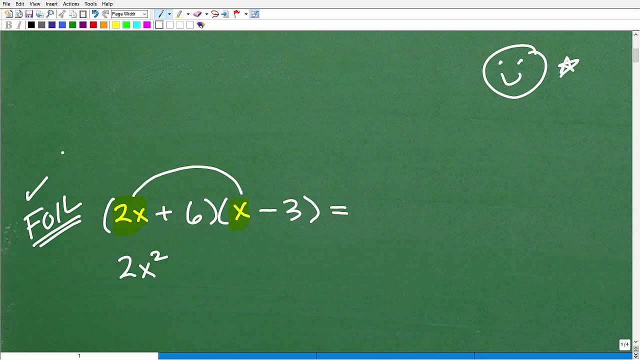 going to be 2x squared. Okay, That's our f. Okay, So that's the first. Now we're going to do the outer. So these are the outers right here. Okay, Boom. So that was the first. This is the outer. 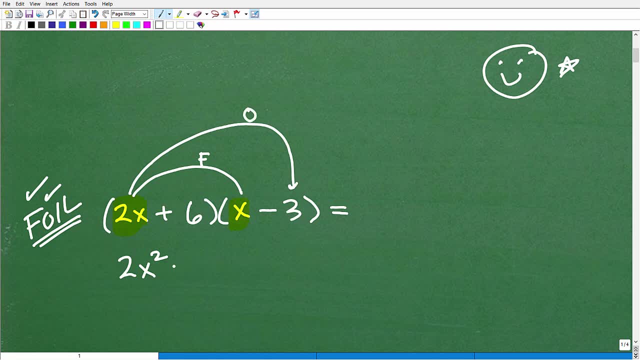 So that's going to be 2x times. This is the negative 3.. And that's going to be what? Negative 6x? So we'll put that there: Negative 6x. And now we're going to do the inner. All right, These are the inners. right there, I'll put a little. 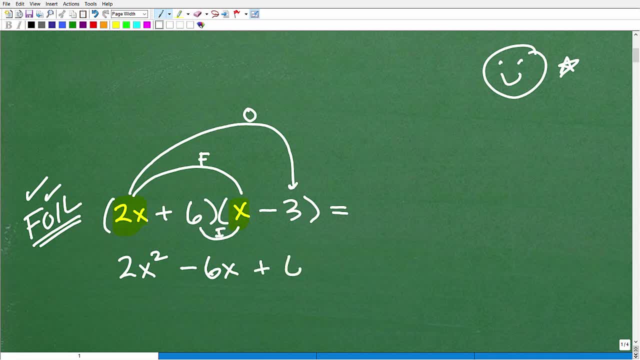 i. So that's going to be plus 6x, Okay, And then we'll do the last, So that's going to be 6 times. These are the last of the terms. 6 and negative 3 is negative 18.. And then we'll go ahead and kind of 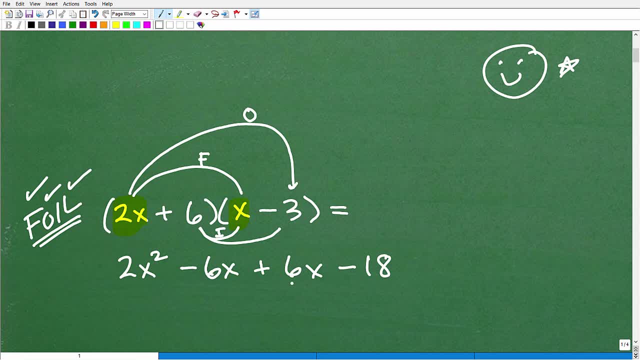 clear all this up. So we have 2x squared minus 6, plus positive Minus 6x, plus positive 6x. These go away. interesting enough, And we're left with 2x squared minus 18.. Pretty interesting right. 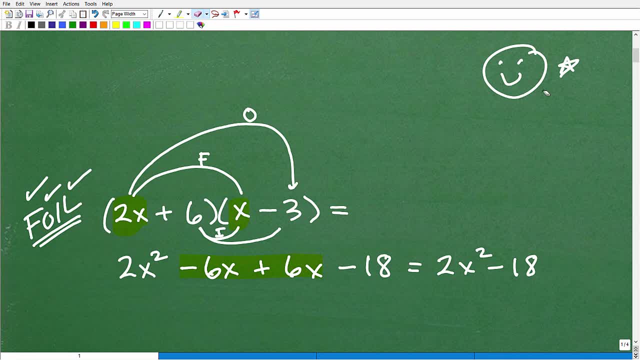 Okay, Now let's just. I'm going to do something here real quick. I'm going to get back to this problem, this one that I did, But I just want to show you 2x squared minus 18.. That's the answer to this. Well, I'm wondering, I'm just wondering how many of you out there can. 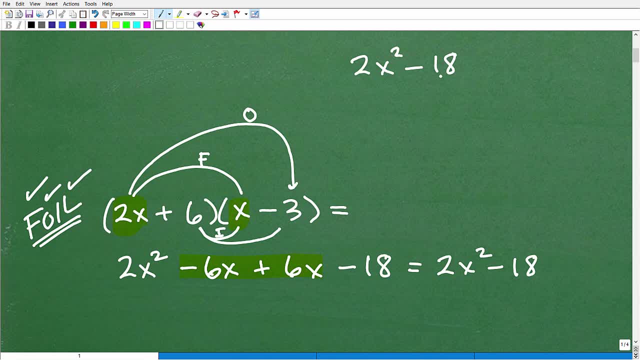 factor 2x squared minus 18? Okay, Have you learned factoring? Well, if you're learning how to multiply polynomials, you probably haven't learned how to factor yet, But you can factor this expression, Okay, And it would look like this too. Well, basically we're doing: factoring is multiplication. 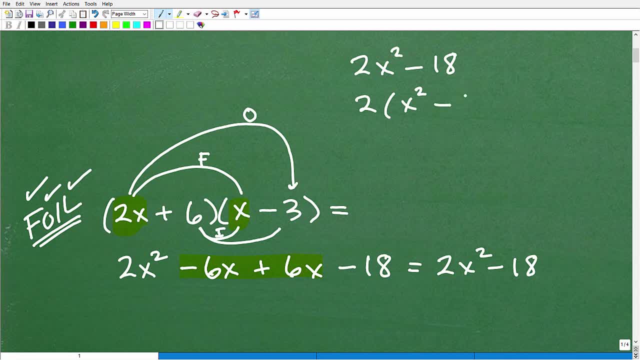 the reverse of multiplication. All right, So this would be 2x Times x squared, minus 9.. Okay, All right, Because this 2 distributed here would get us back to this way, And then this is a situation called the difference of 2 squared. So this is going to be: 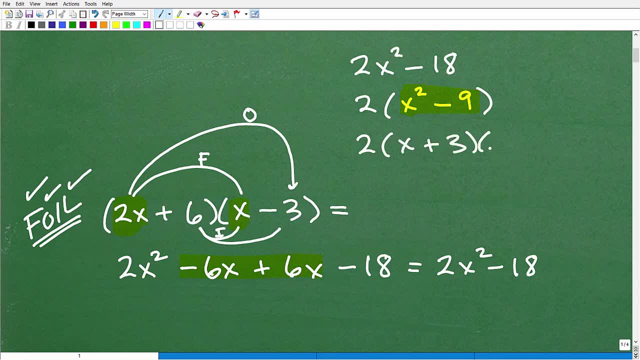 2 times x plus, 3 times x minus 3.. All right, This rule right here: a squared minus b squared. All right, That's equal to a plus b times a minus b. Now, if this isn't familiar to you, 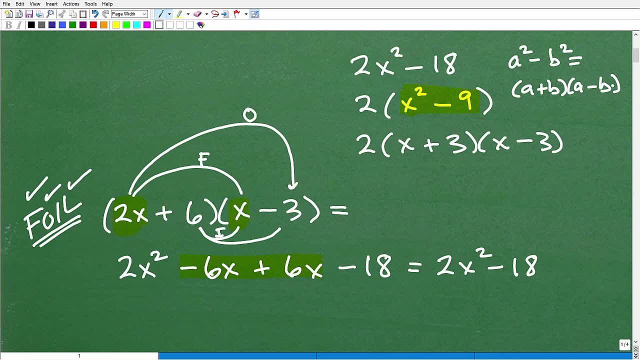 and it may not be. you're going to be learning this. Okay, I'm just kind of giving you a heads up. All right, That factoring is the reverse of multiplication. So that's why we learn how to multiply polynomials- really, really good. 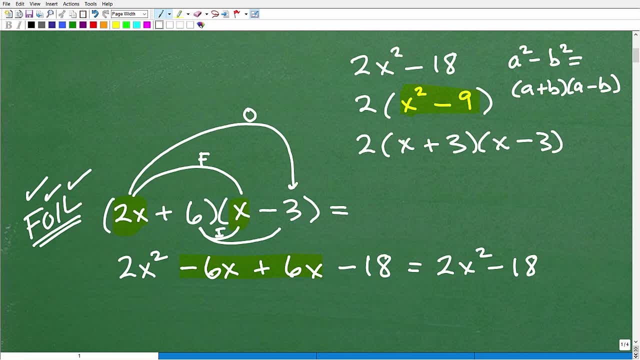 because we're going to have to learn how to factor them. So I'm just showing you a basic illustration of this. And in factoring we do encounter some rules like this. But so we have x plus 3 times x minus 3.. But if I distribute this 2 back into this term, this is going to be 2 times x. 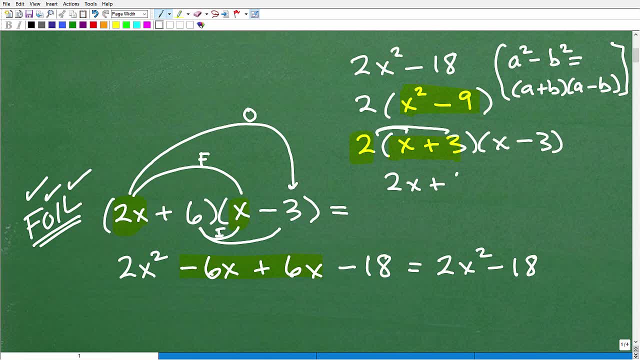 That's 2x plus 2 times 3.. 3 is 6.. Okay, And let's just see if that is what we were trying to. multiply, Yeah, 2x plus 6 times x minus 3.. There, it is right there. So that's just a illustration of factoring And hopefully, 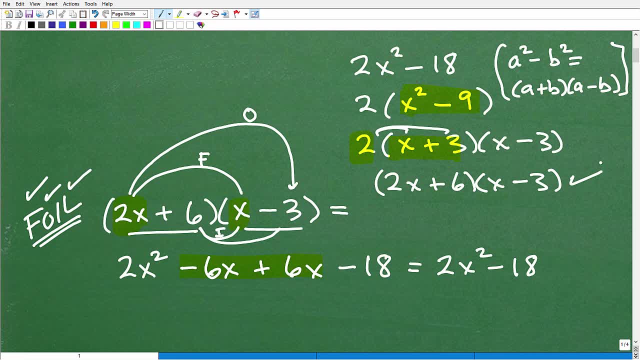 you know, you're kind of familiar with that. If you're not, don't worry about it, You will be learning it. Okay, And I can tell you right now: you can't learn factoring until you understand a multiplication. Okay, That's why this video is important. Okay, But this is 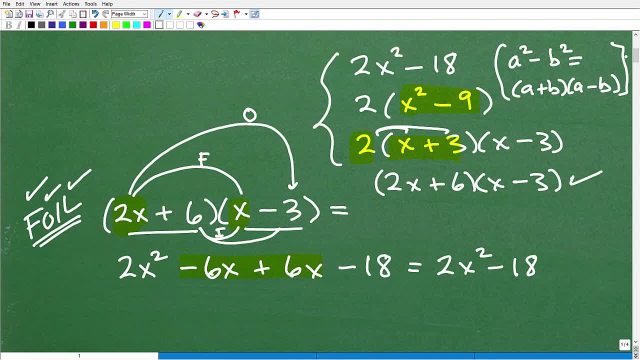 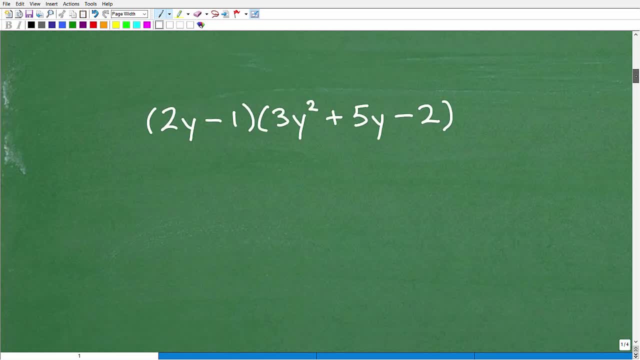 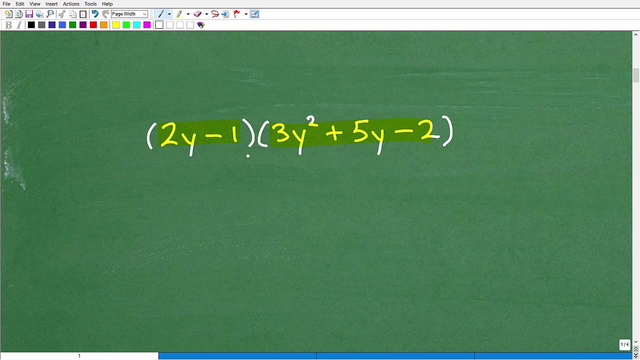 a little preview what you're going to be learning later in another chapter or two in your algebra course. All right, Let's move on to our problem here, Okay. So how do we handle this? Okay, We have a binomial times, a trinomial, Okay. Now what I'm going to show you here is kind of 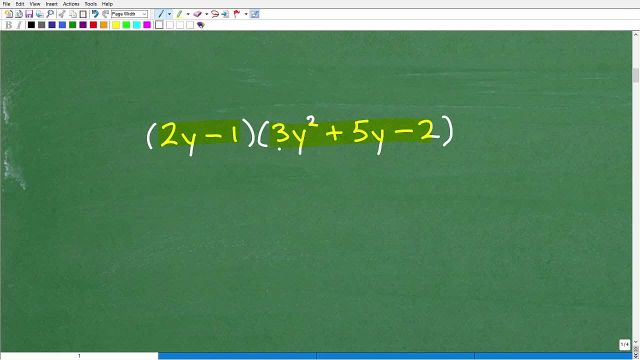 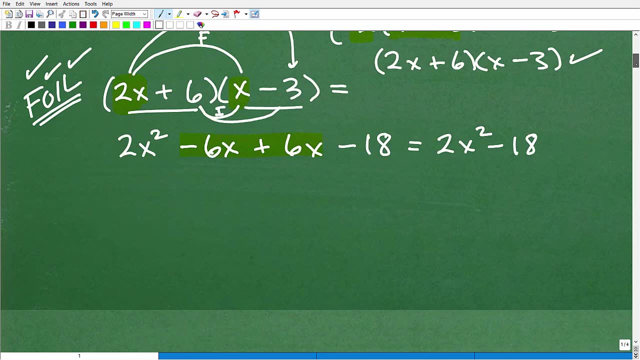 this is going to apply to any polynomial situation beyond the basic situations I taught you. Right? The last problem we ended up with was two binomials. Okay, So when we had a binomial. now binomial has two terms, right? So two things and two things. 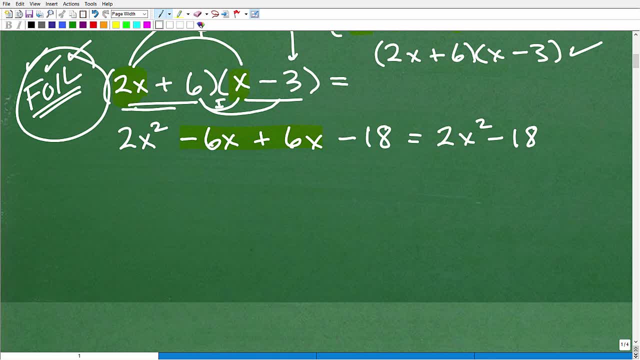 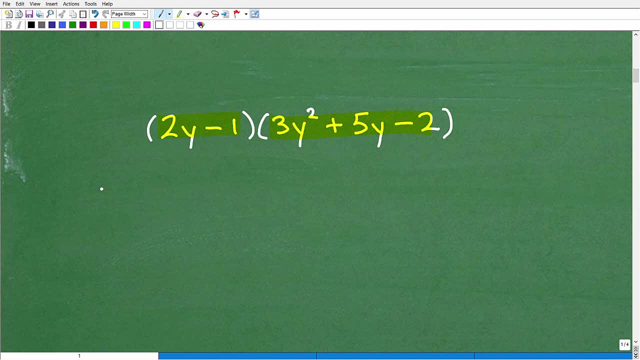 here we can use that FOIL method, But anything beyond a binomial we start getting into trinomials like this: a binomial times a trinomial or a trinomial times a trinomial. We need another method. We don't have a FOIL method, if you will, Okay, But the FOIL method really is kind of. 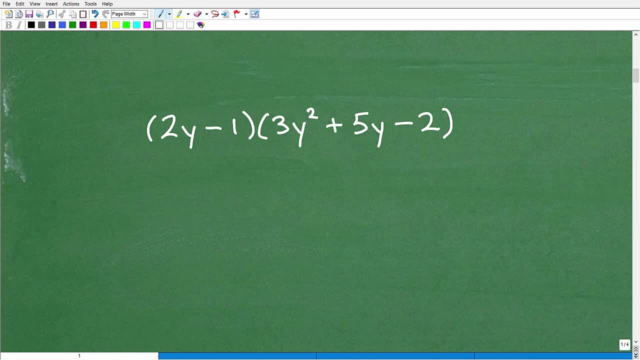 going. it's basically the same thing as what I'm going to teach you right here. I want you to think of this as a basically like doing the distributive property, Okay. So here's how this is going to go. We're going to start right here- Okay With this term- and we're going to distribute this. 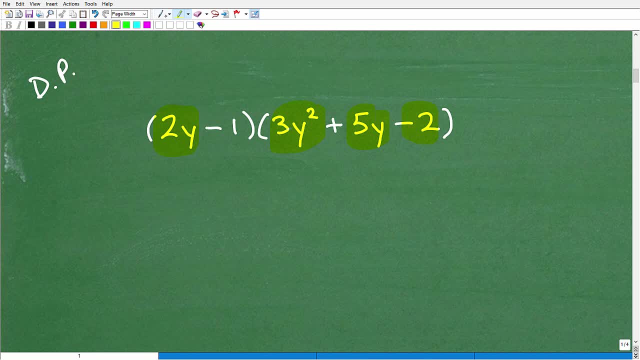 term to all of these guys. Okay, And then let's go in and just start the problem, And I think you'll see understand this better. you know as I do it. Okay, So we'll start here and now we're going to distribute Boop, boop and boop, Okay, So well, what I mean? 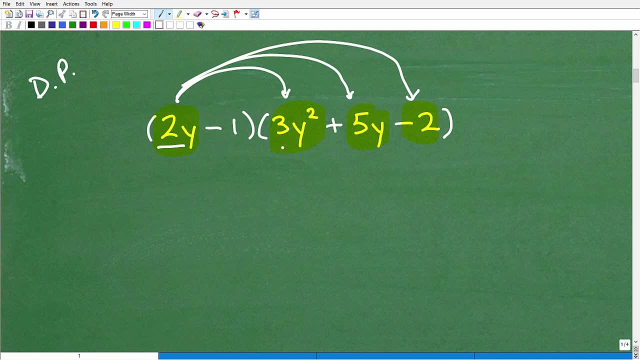 we're going to multiply, So 2y. we'll take 2y and we'll multiply it by 3y squared, All right, So that's going to give me 6y cubed. Okay, Got to be very careful y times. y squared is y cubed. 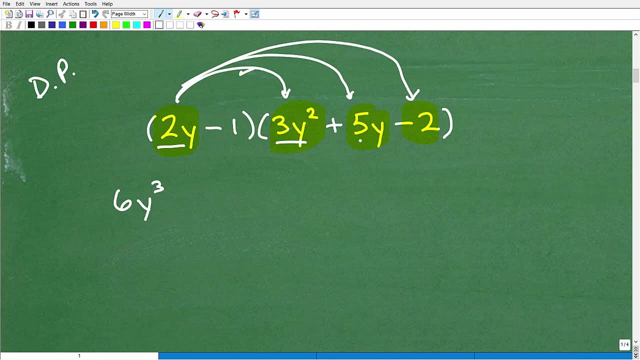 All right, So that's that. Now we'll take 2y and we'll multiply it by this positive 5y, So that is going to be plus 10y squared, All right. So again, I'm going to start off with this: 2y times this 3y squared, That's 6y. cubed, 2y times 5y is 10y. 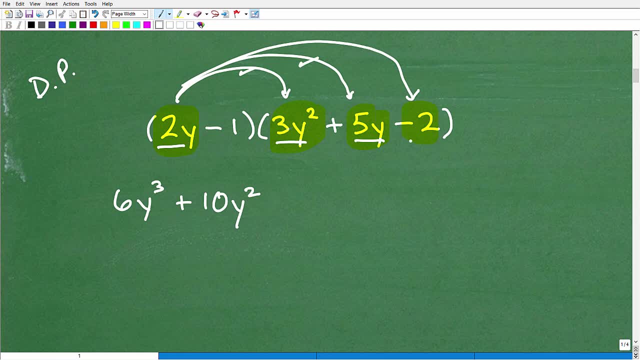 squared. Okay, We did that And I will do 2y multiplied by negative 2. And that'll be a negative 4y. Okay, All right. So you're you know. maybe you know all you out there are like: 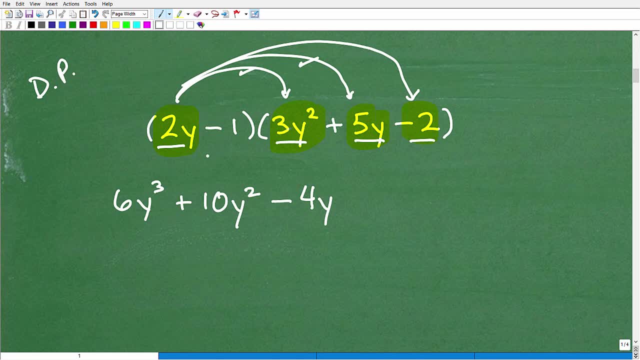 yep, I get that, So let's continue on Now. here's how this distributive property kind of technique works. Once you've used, once you've uh kind of ran out of things to do with this first term, All right, You keep going to the. 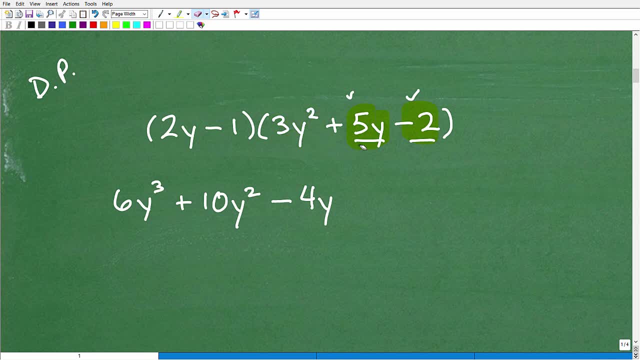 right, In other words, I'm going to erase all this. Okay, So I took this 2y and I distributed to all these things here and I got these answers. Okay, I'm done. but you're not done yet, because what we need to do is this part of the problem: this first polynomial, whether it be a binomial. 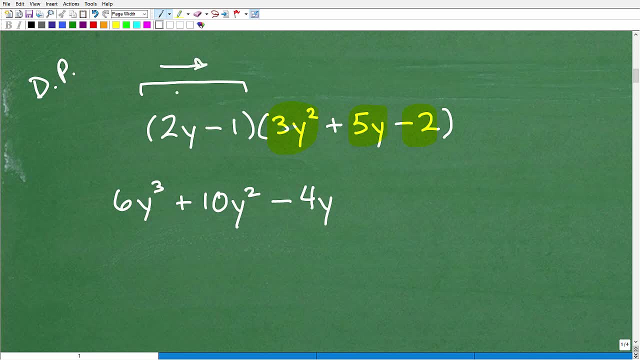 or trinomial, it doesn't make a difference. We have to keep going uh to the right, to all its little uh, whatever terms it has. we have to do the same thing. So we did 2y, So now we have to move on to the next term. that uh is in this particular. 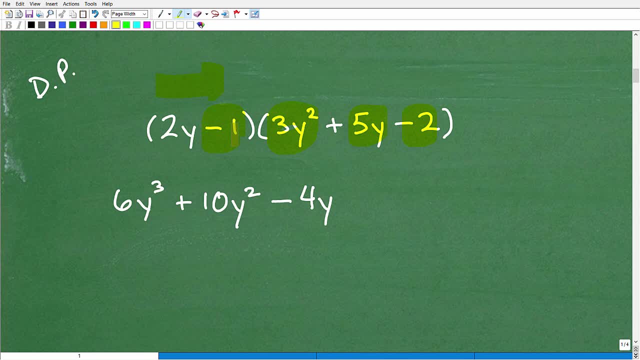 polynomial. Now, if it's a binomial, the next thing to do is negative one. If it was a trinomial, we do the middle term and then the last term, right, So we're going to go ahead and do the. 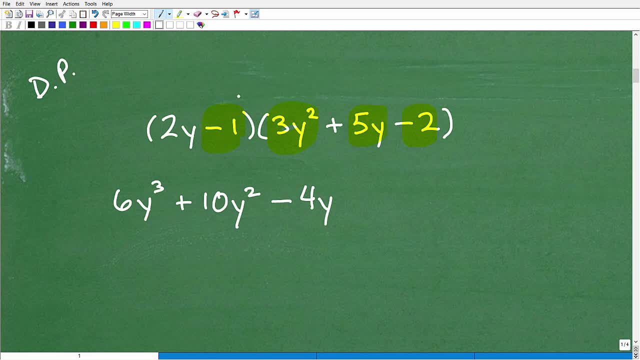 exact same thing, but this time we're going to distribute this negative one to each of the terms. Okay, All right, So let's go and do that now. So negative one times negative 3y squared is negative 3y squared. Now we have a negative 3y squared. I can write it right there. but notice I have. 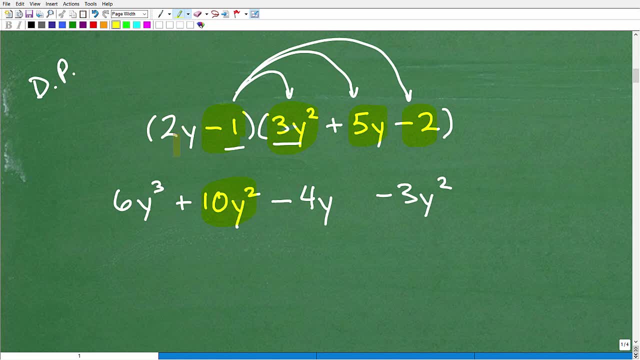 my y squared term right here from the previous step. Okay, So what you'd like to do, right? When you get the same powers negative one times 3y squared, put it like in a column. It's just going to be easier to combine. 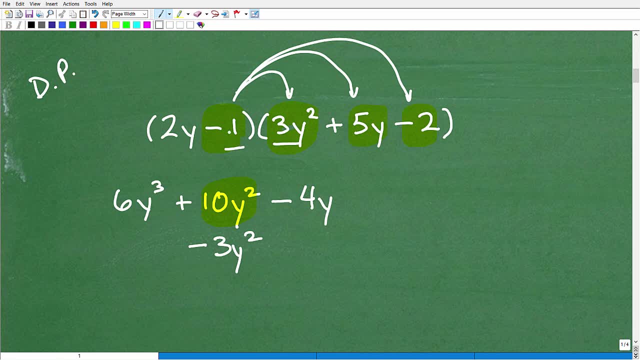 Terms: negative 3y squared. All right, Now we're going to take this negative one. We'll multiply it by this 5y. That gives me negative 5y, And I have my y term right here, So I'll line this up. 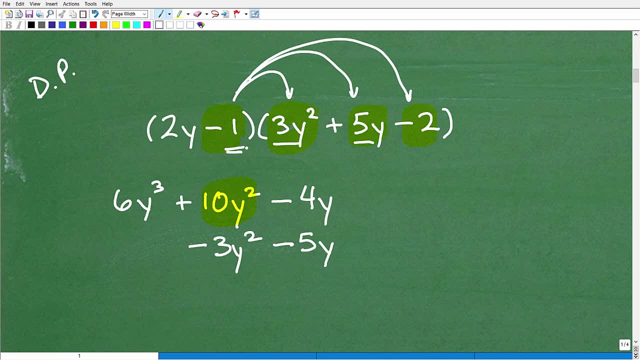 negative 5y. Okay, And so I'll take my negative one, multiply it by this negative two, That gives me positive two, And I could just write that over here. Okay, So now I'm done, Okay, Uh, distributing uh this negative one. Okay, And now is there any more terms? 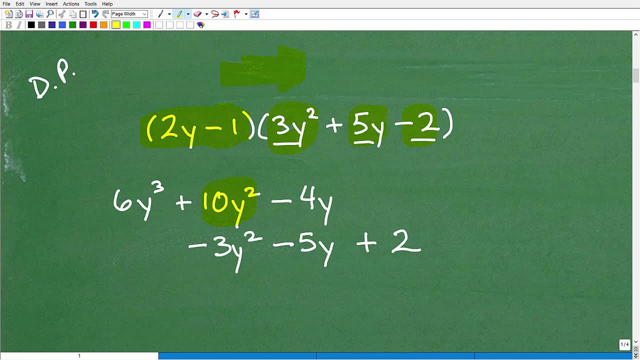 There was more terms in this polynomial, I would just continue to do the same thing. but we are done. We distributed this and we distributed this, So now I just have a bunch of terms I have to add up. This is combining like terms. Let's go ahead and do that now. 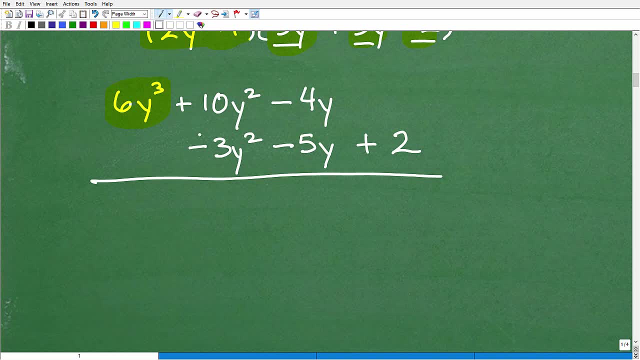 All right, So I have six y cubed. Is there any more y cubes? Nope, Uh. so we'll put six y cubed and we want to write this in standard form. That's the highest to lowest power. Okay, So six y cubed, that's our highest power. There's no more y cubes. So that's it. We could just cross. 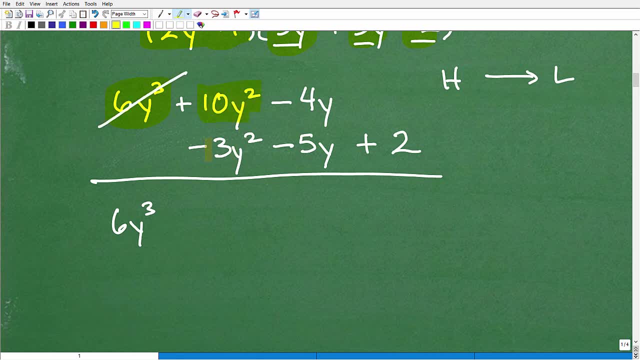 this guy out. So we have 10 y squared and negative three y squared. I can add those by adding the coefficients and that's going to be a positive seven y squared. Okay, Remember, highest to lowest power. I'm going to do my y squares next. I can just get rid of them. Now I'm going to move on. 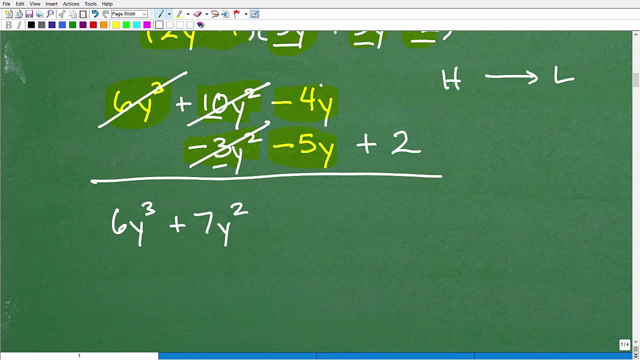 to my y's, That's my, or y to the first, That's my uh x power. So negative four and negative five is negative nine y, And then finally, I just have this lonely two here. We've got to go ahead and add him to the end of this polynomial And that's it. 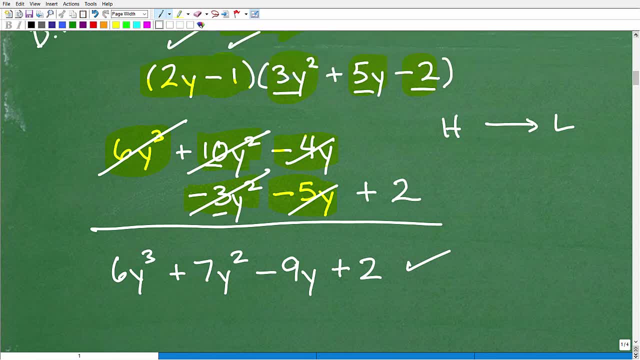 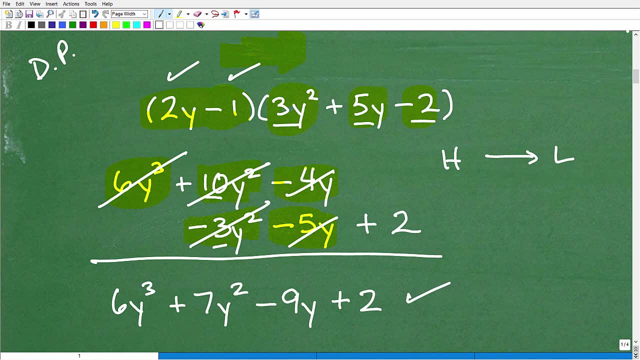 Okay, This is the product of those two polynomials. Now, I like this uh technique. This is the distributive property technique. This is very, very good. Now, sometimes this is referred to as, like, the horizontal method. Okay, So some of you out there are like, Oh yeah, this is the. 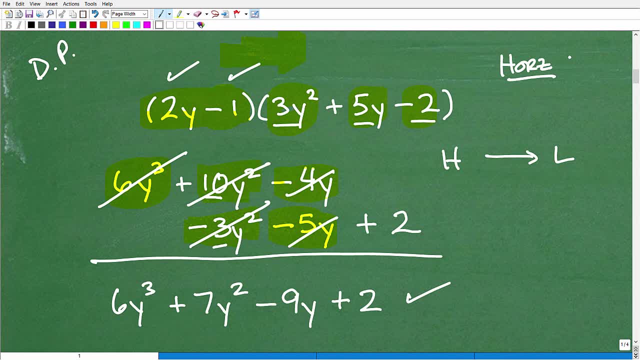 horizontal method. You're absolutely right, It's a horizontal method, but really it's it's kind of a spin on the distributor property. Now there is another technique. Okay, I'm not going to do it, uh, in this particular problem, but I'm going to just kind of quickly show you. 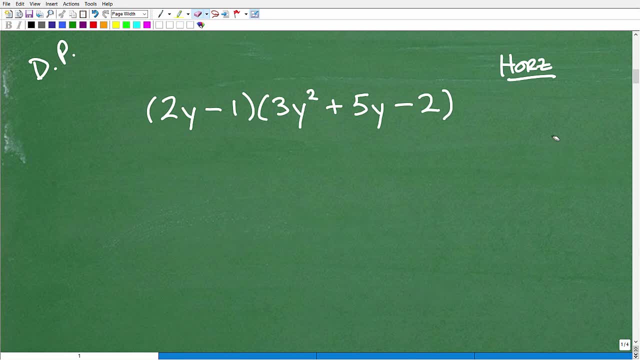 how you set up, uh, for something called the vertical method of multiplying, um, uh, polynomials. So your teacher might, um ask you to do this. So what we're going to do is going to put our biggest polynomial here. So we're going to put our biggest polynomial here. So we're going to put. 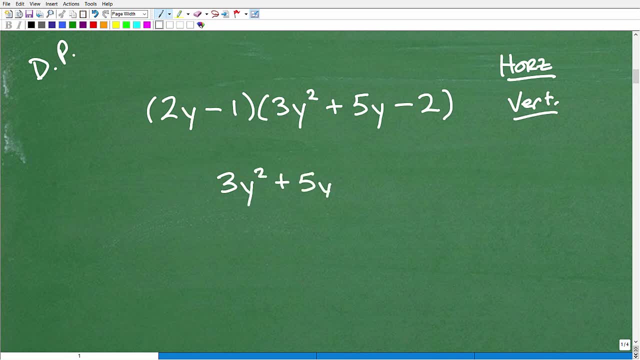 three Y squared plus five, Y minus two, And we'll put our smaller polynomial just like regular division, like an arithmetic. We have two Y minus one and you just draw a little line like that. So this is vertical, right? So we have things lined up in a vertical manner And here you start. 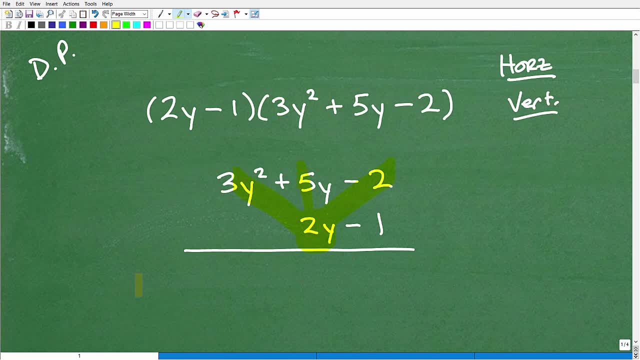 with this and you're going to multiply to all these terms. Okay, You're going to get your answers: Boom boom, boom, boom boom And notice we're doing the exact same thing as a horizontal method. Okay, Right, Or the distributive property, but I like the distributive property because 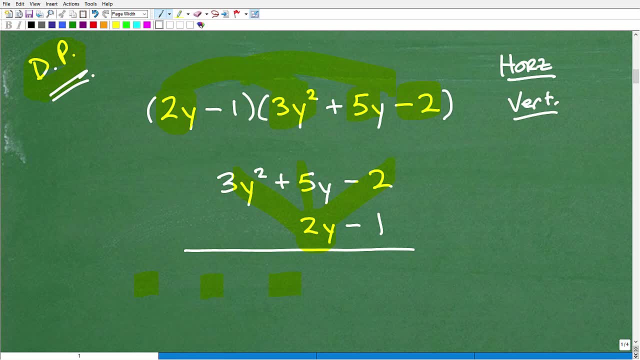 once you understand the distributive property, then you can kind of think of: you know, that's what you're actually doing here. Okay, But this is an example of the vertical method. And then, once you're done with this, uh, you move over to the next one. 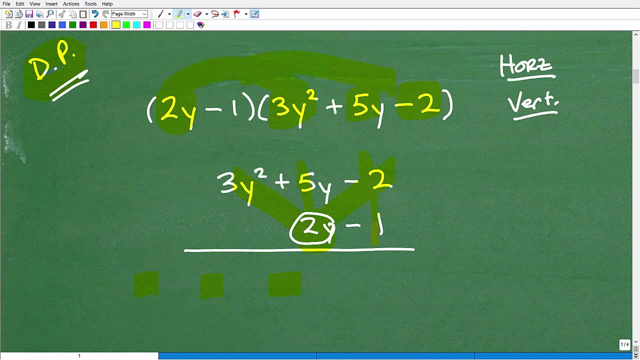 or you can start with the negative one, uh, and move over to the two Y doesn't make a difference, You'll do this. You'll get your other terms- boom, boom, boom- And you'll get the exact same answer as we got, uh, you know, previously, when I was showing you the distributive property or the 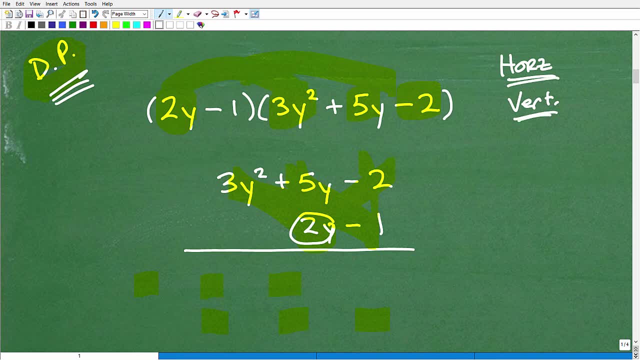 horizontal method. So you're going to start with the negative one and move over to the two Y Again. there's always, you know, a spin on these names, depending on you know your textbook or how your teacher references them. but your teacher may have a particular preference for they like. 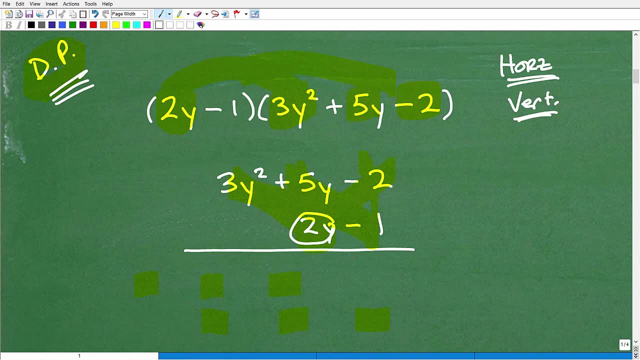 you know, for how they elected um you to learn this. Okay, So you know, follow their guidance, But for me, I think, uh, this horizontal method, which is really again, uh, a spin of the 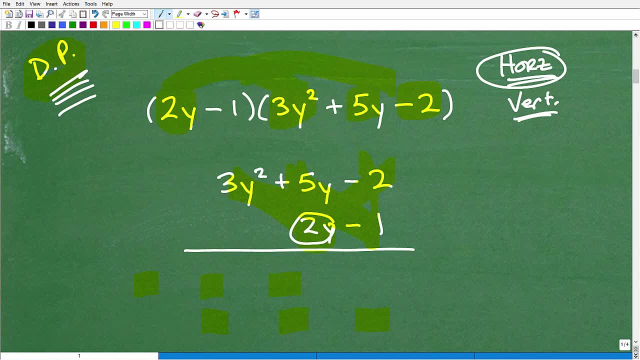 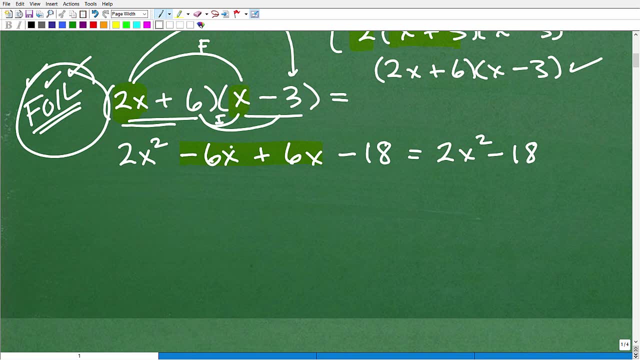 distributive property is, um, the easiest way to remember this because you know, when we do problems like well, like the foil method, we're going to have to remember this because you know that's kind of like the horizontal method. Okay, You're not doing a vertical method, or you're doing. 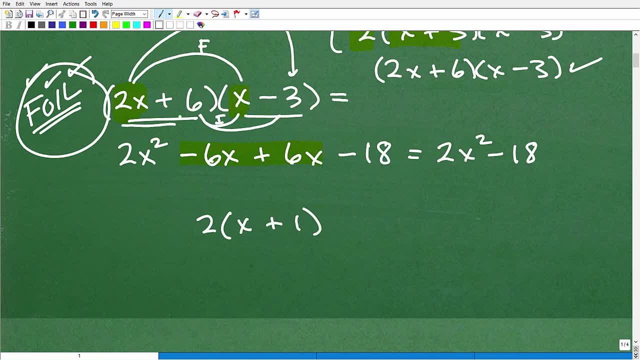 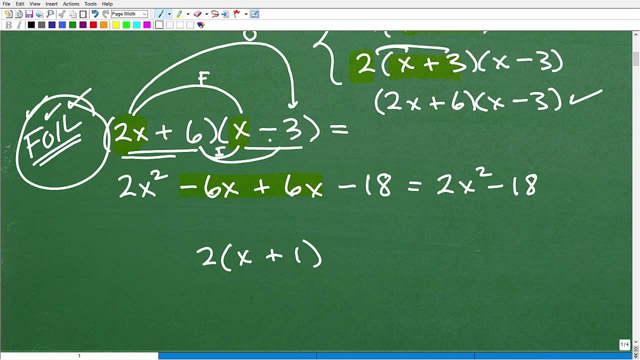 problems like this. Again, these are like an outtake of the distributive property. If you look at the foil method, it's really basically the same thing as I kind of taught you. Okay, It's a binomial times, binomial, binomial. but yeah, we have this nice little term, foil. and believe me, 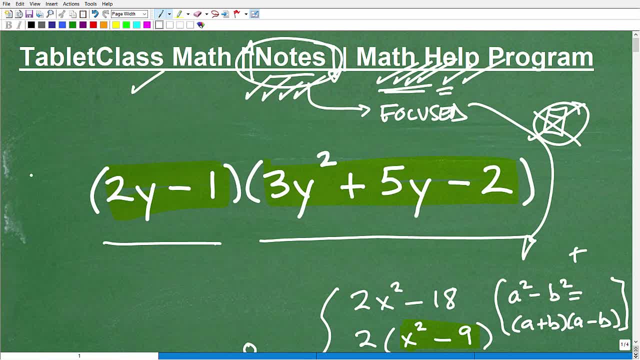 that foil term has been around for a long time. I even remember that's probably one of the few things I remember from high school algebra, way back in the eighties, where you know people had these Mohawk, uh haircuts and stuff like that. Yes, You know we were uh cool way. 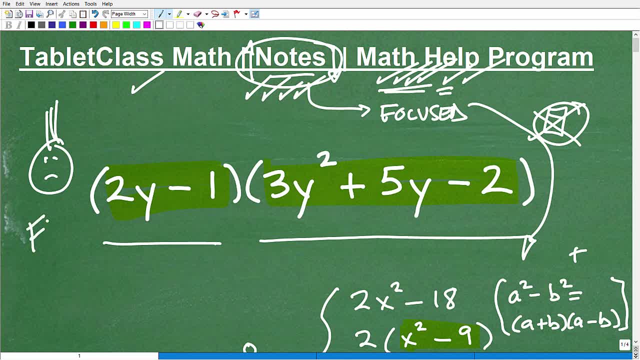 back in the eighties, but I do remember somewhere in the recesses of my memory, learning about the foil method. Okay, I was probably pretty distracted. Uh, maybe my best friend with the Mohawk was talking to me at the time, but I do remember that. So I mean, this foil technique has been around. 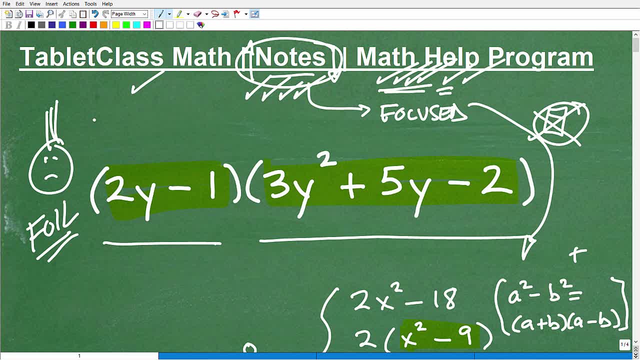 for decades. Who knows, maybe your grandparents even learned it. but uh, you know, acronyms are good, but we need to know that it's like that's a special case Scenario. All right, Okay. So if this video was helpful, if you're like: wow, you know. 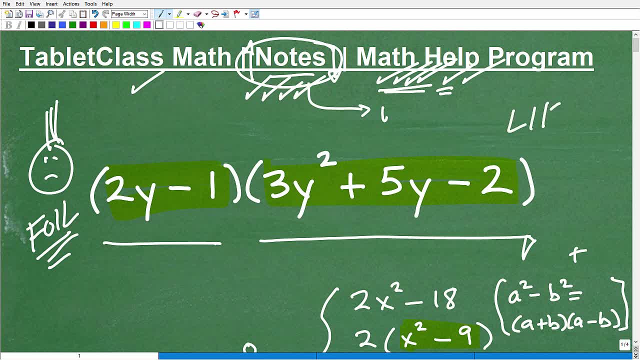 I really learned a lot from this. Well then, please consider smashing that like button. That would definitely help me out. And, uh, please consider subscribing. Okay, If you like my teaching style. well then, that's, that's excellent. My, my passion, my goal is always to try to.